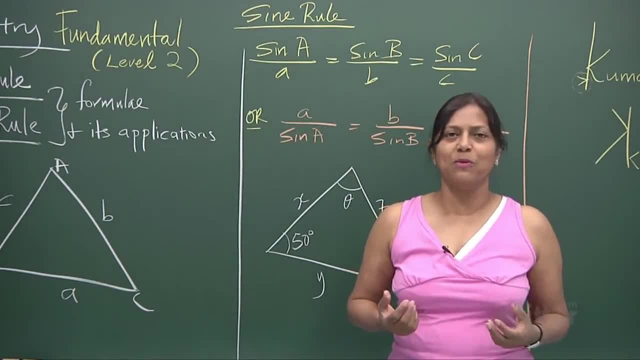 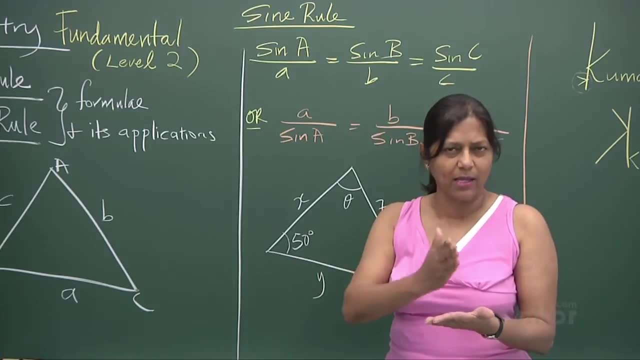 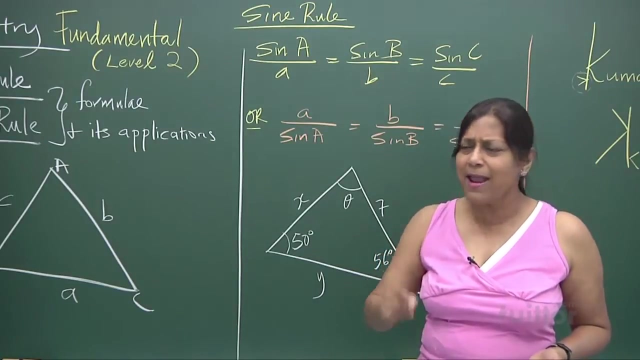 And all these fundamentals will make your trigonometry so much easier. And once you look at the sum, you can diagnose it so fast and so accurately and you can give the right treatment. That's when you become like a max doctor. All right, All right before we start lessons. are you charged? Are you feeling comfortable? 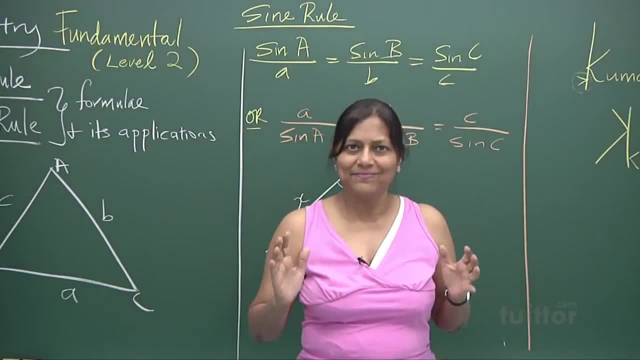 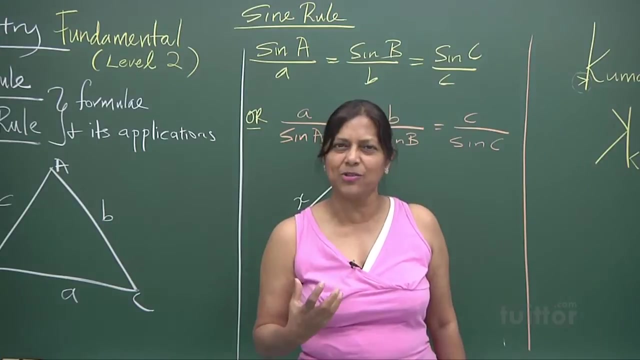 If you are, please loosen up and just be ready. It's something not really difficult. We're going to learn on sine rule, cosine rule and its applications And that these rules, these principles, these applications will help you a lot in solving lots of the trigonometry. 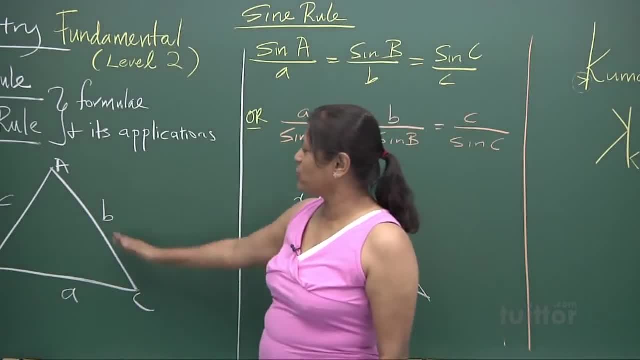 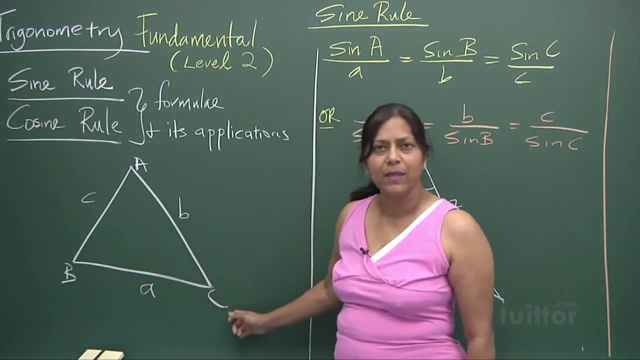 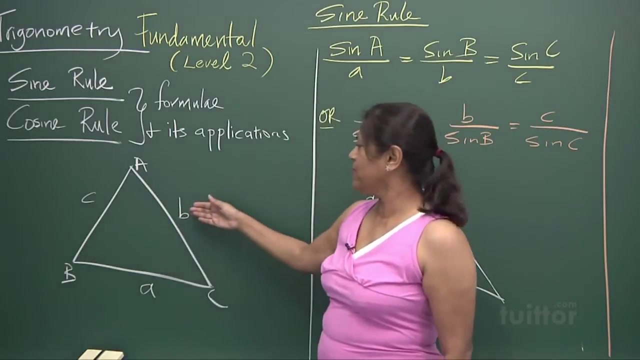 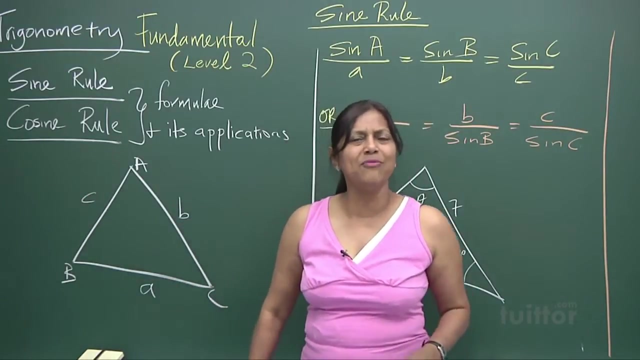 sums. Now, if you look at this triangle, a triangle has three sides, right, I call it triangle ABC. And to face the triangle A, we call it side A. To face B, this is the face B. To face C, I call it C. But you got to know there is a relationship between the angle and the 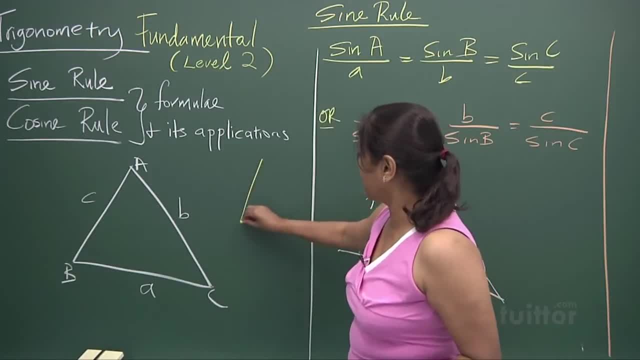 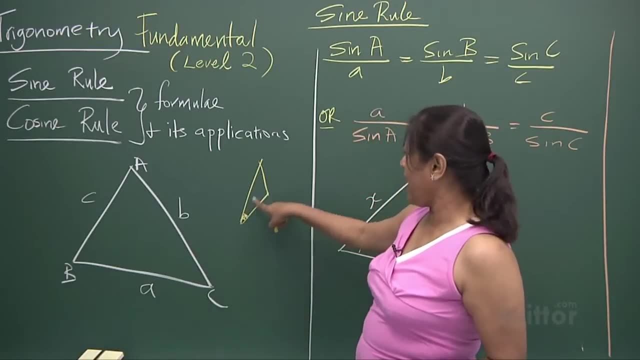 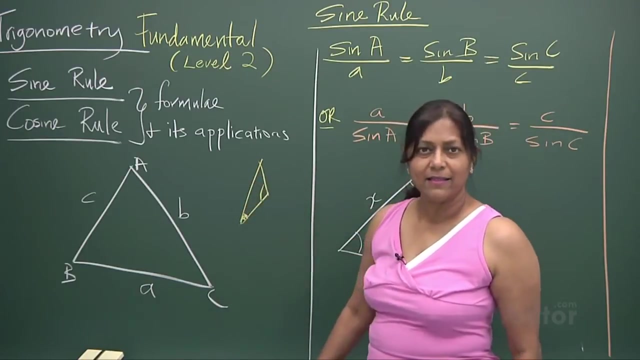 side. Okay, if I have a triangle like this, you can see that this angle is really small. the smaller the angle, the smaller the side. if this angle is big, so it faces the bigger side. are you clear? all right now you can see if I increase the angle. I. 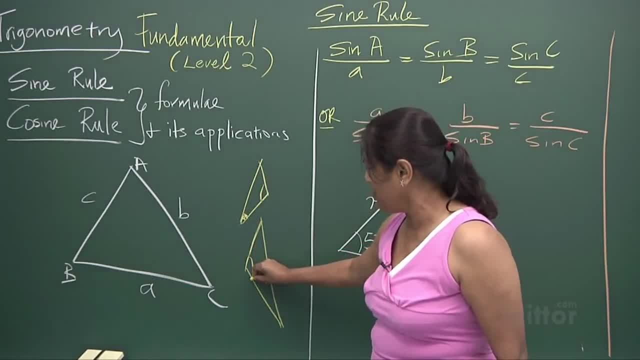 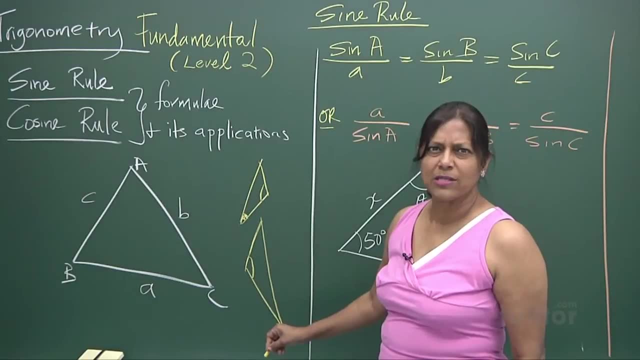 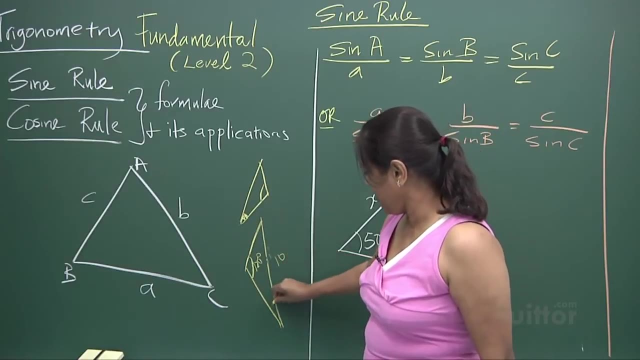 say, ooh, this angle grew and you see the side growing. so there is a relationship and when you do your sum and you will see if this angle is 120 degrees and you get 10 here, and this angle is maybe 20 degrees and you get a side 12. for 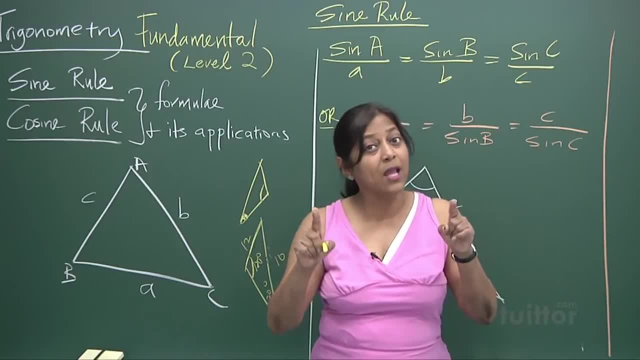 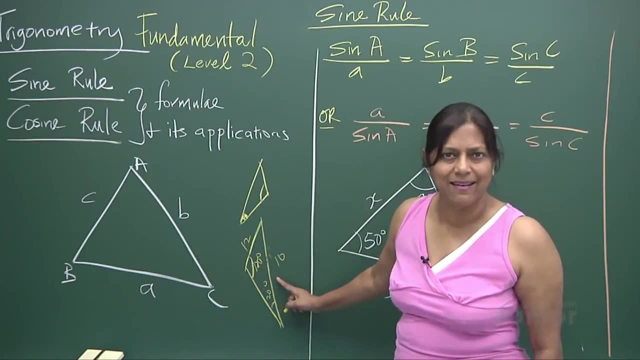 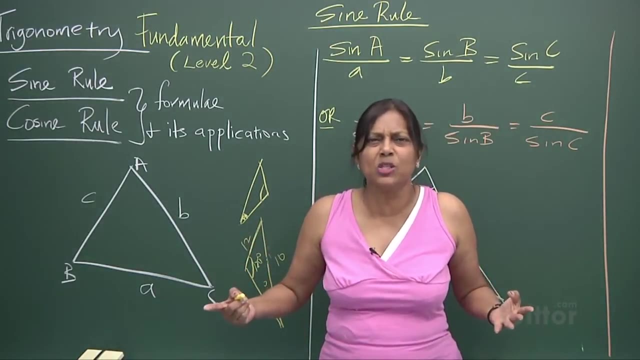 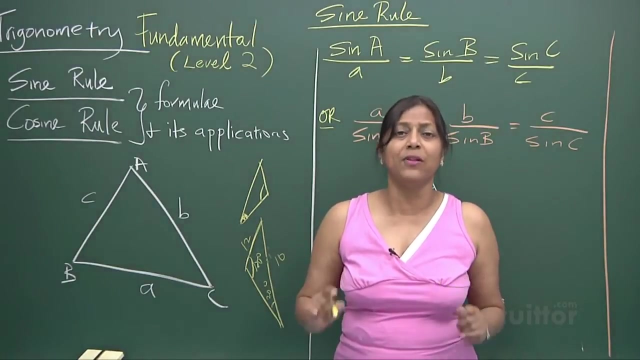 example. then you tell yourself something cuckoo took place. all right, because when hundred and twenty degrees is facing 10, how can 20 degrees face 12? maybe two degrees, it may be three, it may be much smaller, all right. so this is just an intellectual guessing of seeing the level of accuracy of your answer. all 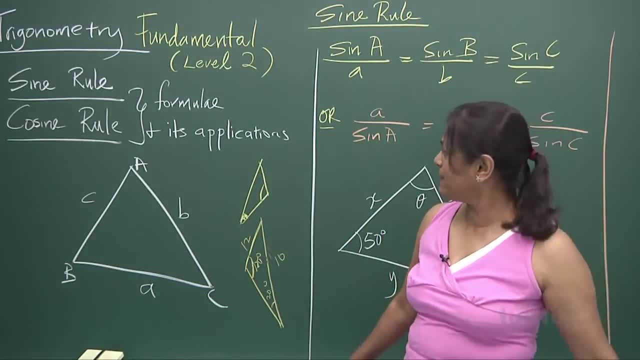 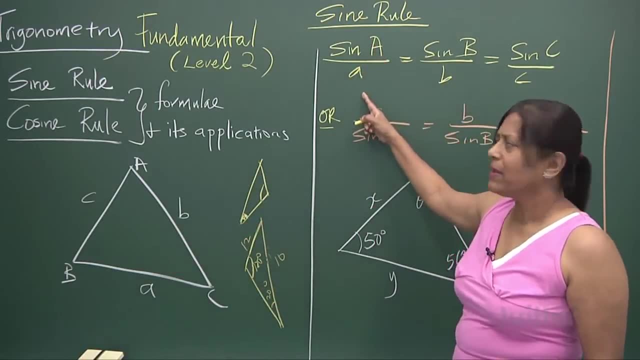 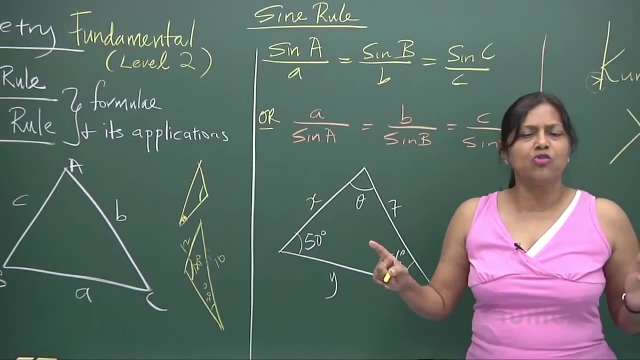 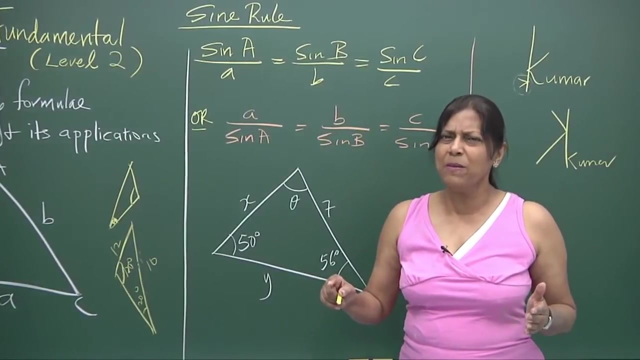 right, every calculators with you, because we're going to apply this. okay, now, when we have a triangle, ABC, now, sine a over a is equal to sine B over B, equal to sine C over C. now, whenever you draw any triangle, you will see that this amazing relationship holds. all right, you will be. 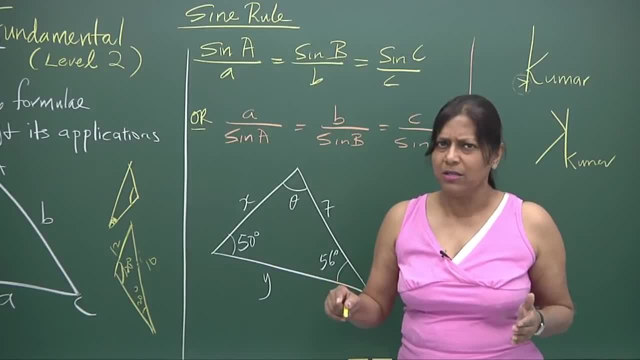 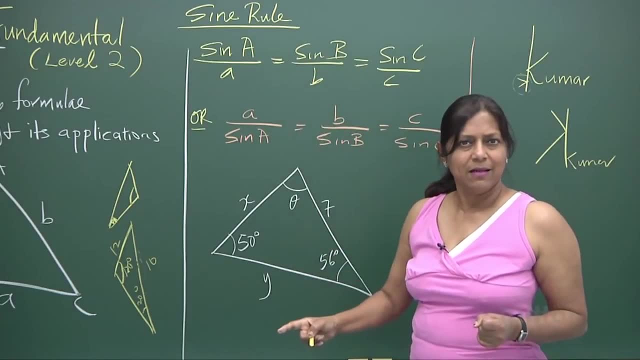 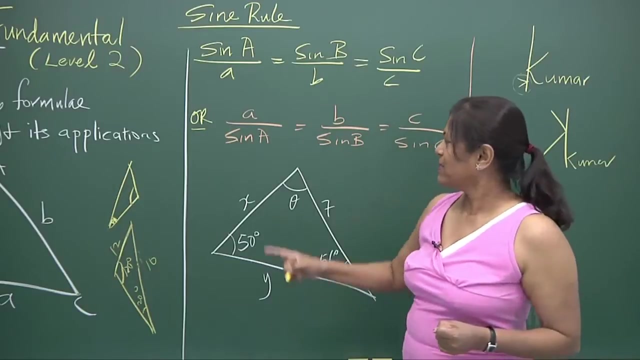 surprised and I will show you because I don't want to bullshit. I want you to be convinced by what you're doing. there is this ratio that is discovered, all right, and this beautiful ratio stands for all triangles. so sine a over a, sine B over B, sine C over C. but the very important thing is that you have to know that this is an 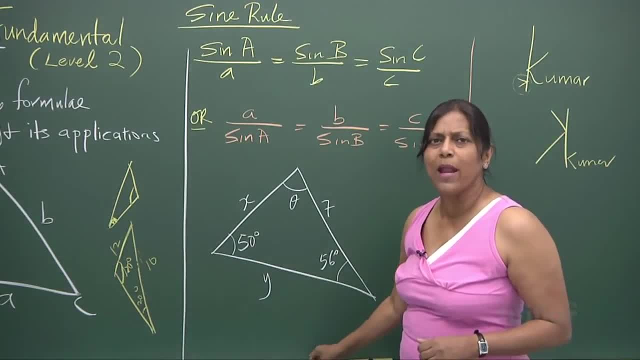 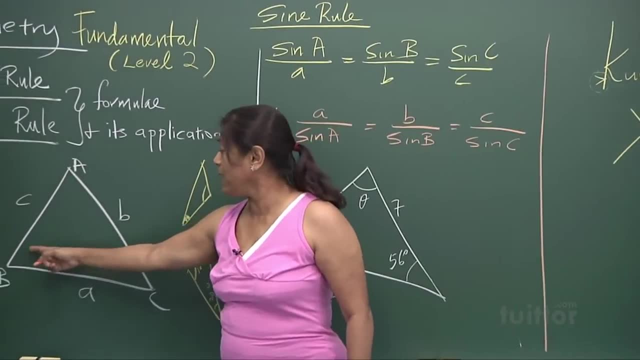 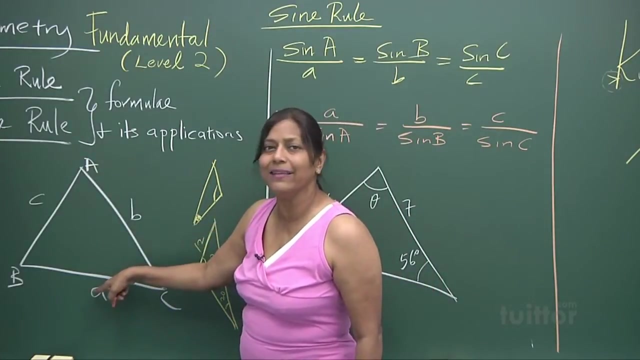 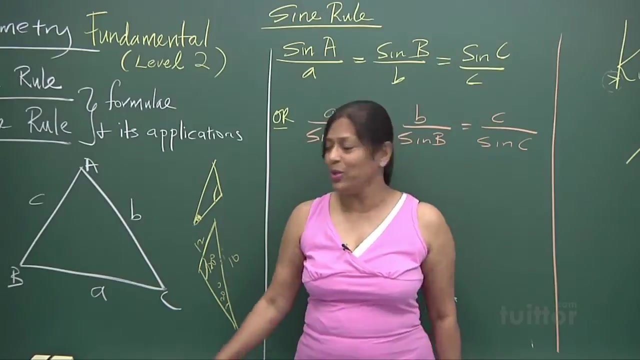 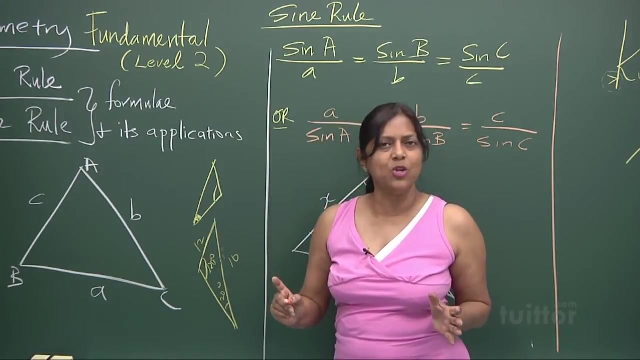 angle B. you know so the angle here. so now I will just put perfect, can you hear me? okay, this isn't the right angle here. and break it to the side now. the other important thing about here is important thing is that when you use sign rule, you must have a given pair. all right if any one. 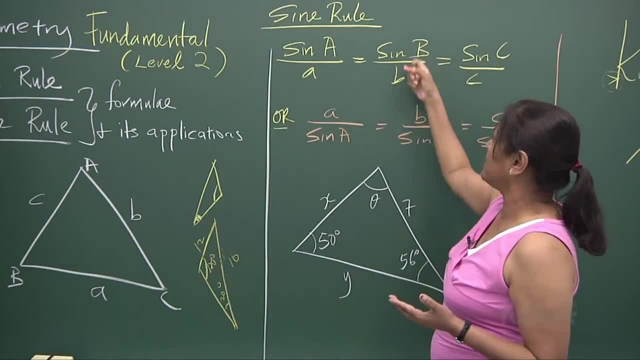 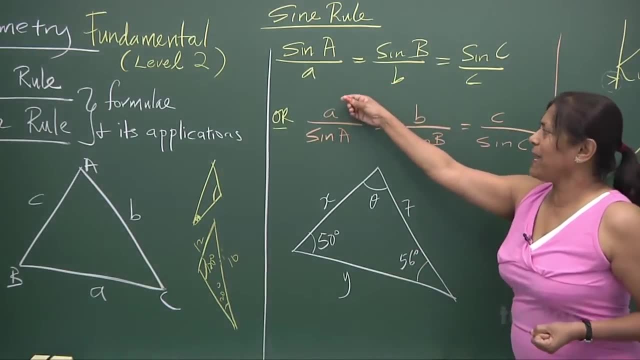 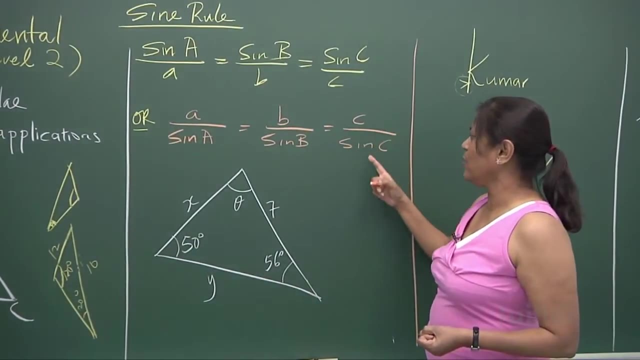 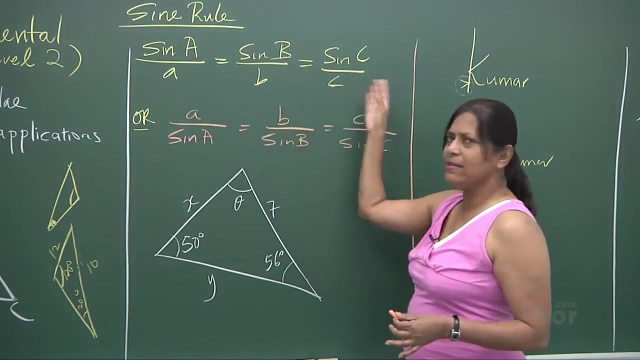 given pair is given, and then, if any of this is given, you could solve it. i'll show you more as i go along. now. this sign rule could be expressed as a over sine a, b over sine, b c over sine c. isn't it very simple? all right, it's either angles over the sides or the sides over the angles right. 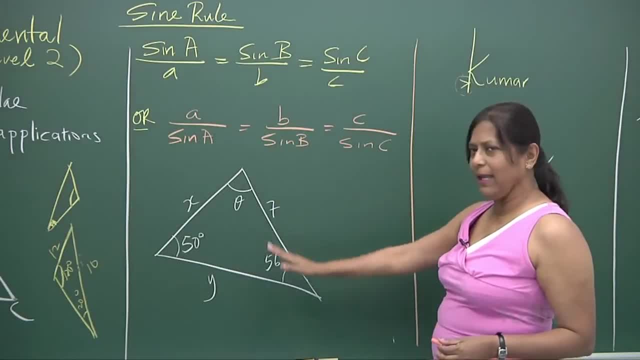 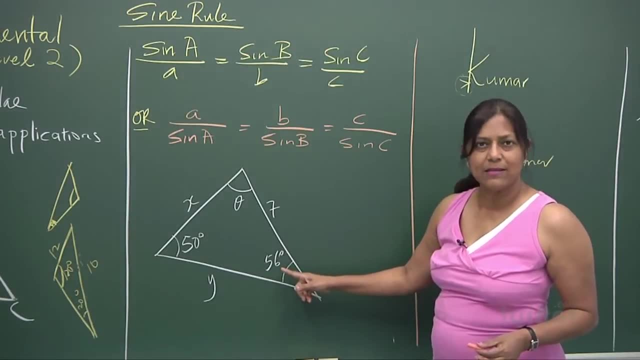 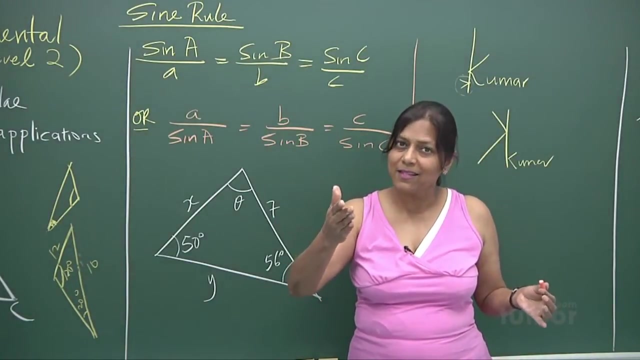 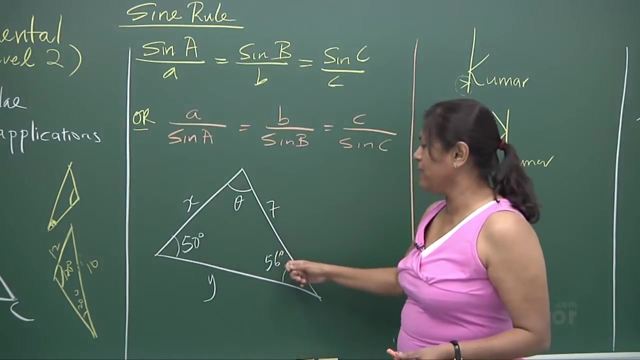 really simple. now let's look at this. hey, now we've got a given pair right and you'll get 56 degrees. just ask yourself: will it be bigger than seven or less than seven? yes, i hear you, your inner voice. it must be more than seven. all right, and if you know these two angles, 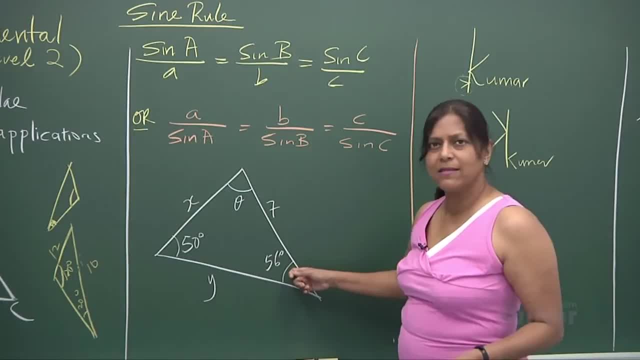 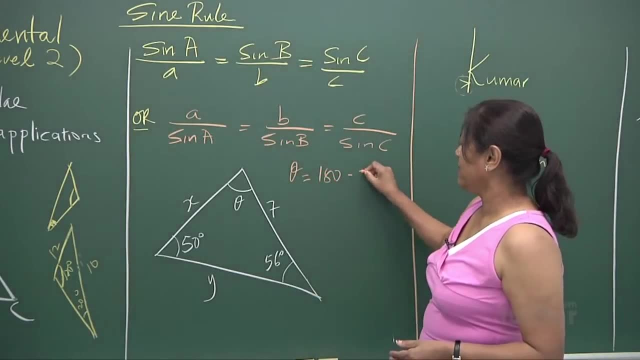 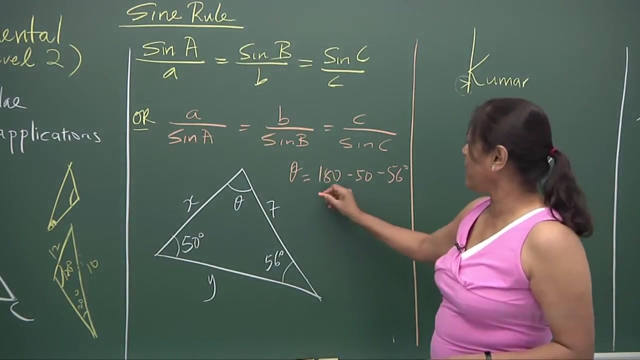 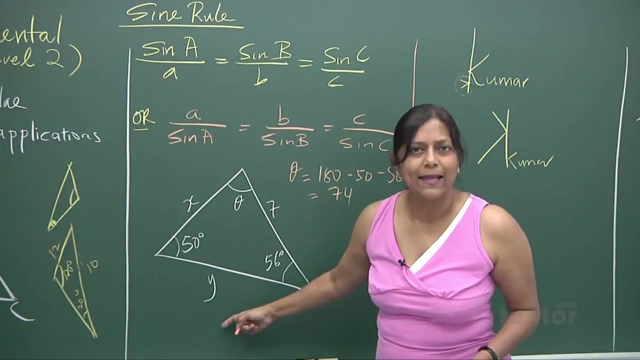 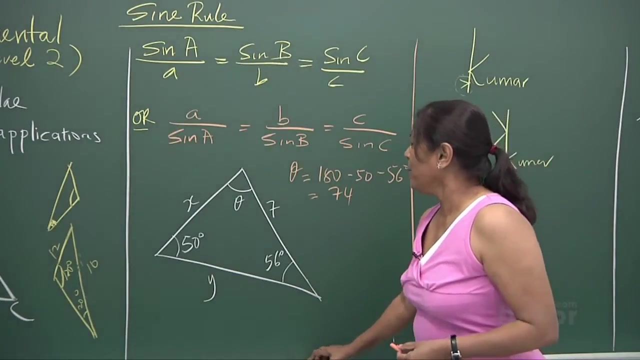 can you find out theta? this is 106. angle sum of triangle will tell you that theta is going to be 180 minus 50 minus 56, that's 106. so if you take away you get 74 degrees. so of course y is going to be the longest side of this triangle. now from there we could apply: i'm going to erase. 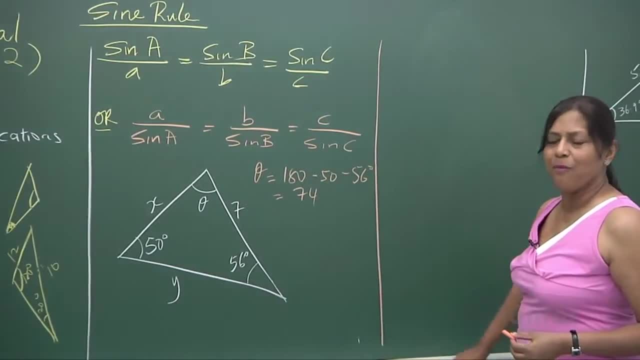 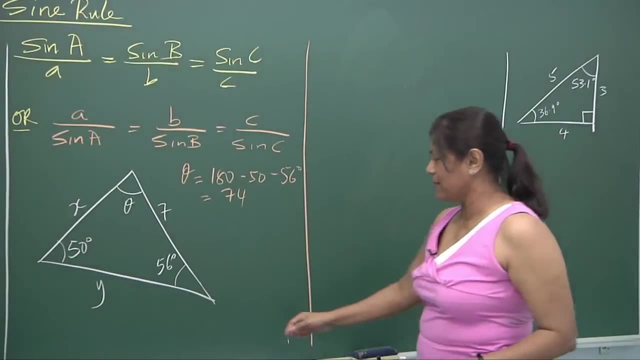 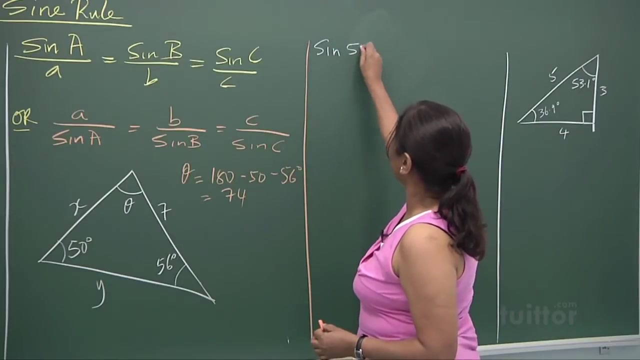 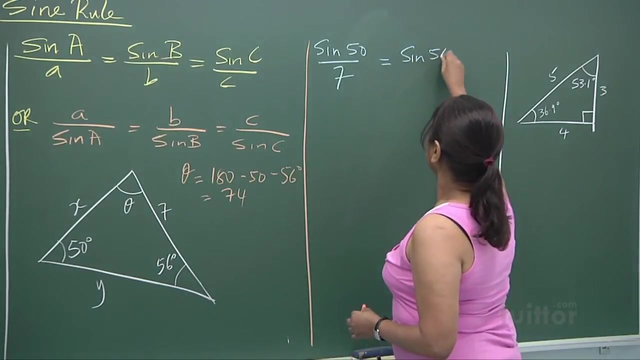 this kuma off and we're going to apply the formula to solve for x and y. how do you go about that? let's put in the formula. we've got it. we said a is sine 50 over seven. all right, is equal to sine 56 over x. now the amazing rule here is that we know we can cross multiply. 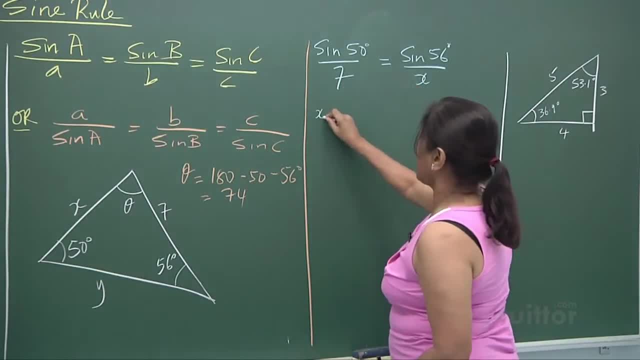 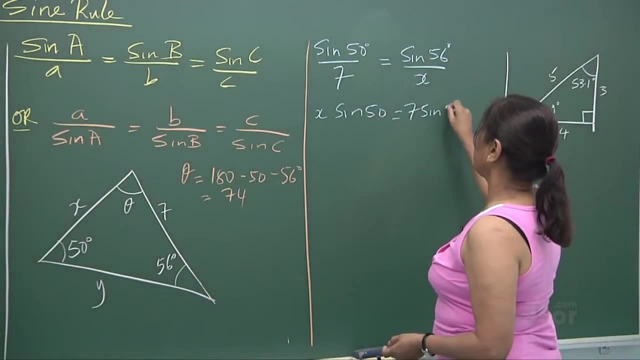 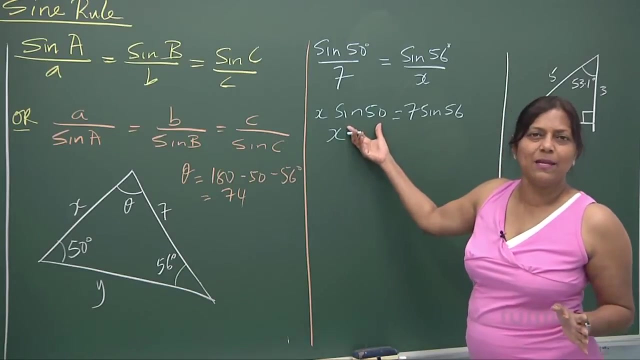 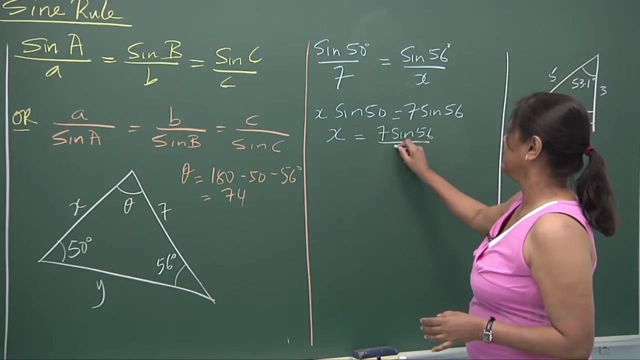 and so you can bring your x up, you get an x sine 50. and you can bring your 7 up, you get a 7 sine 56. now all you need is x. hey, and this is an attachment times. bring it over and you would get that lovely answer right. so can we try, please on your calculator. 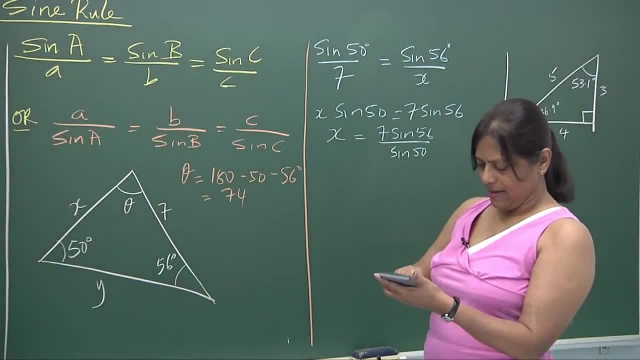 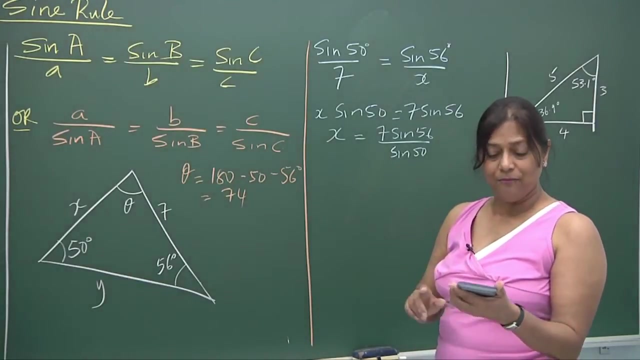 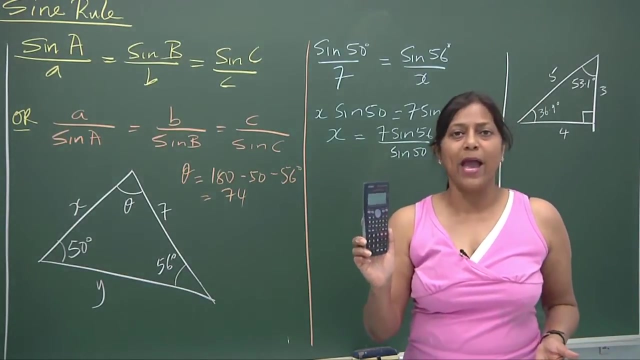 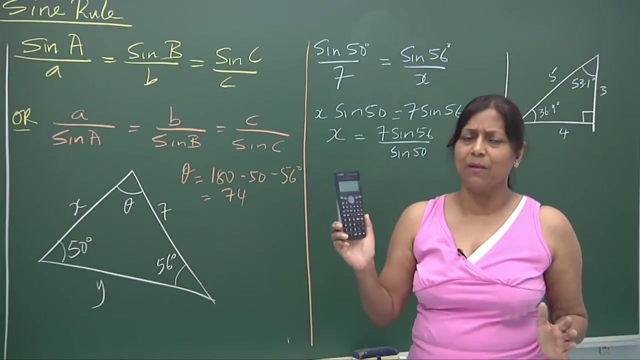 7 times sine 56 degrees, answer, and you divide it by sine- 50 degrees, all right, and you get what you get. is you get 7.5756? now in your school they may want your accuracy to three significant things, or three, or maybe two: decimal place or the nearest angle, or whatever they might, they will. 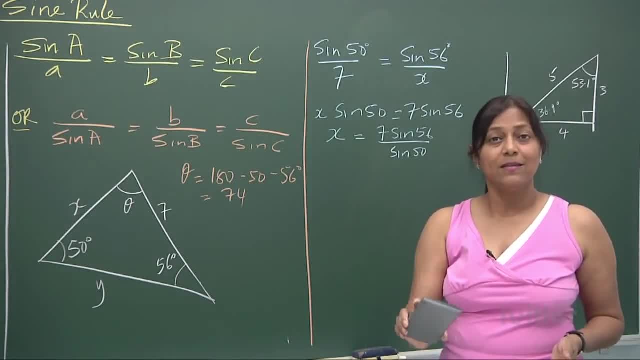 specify. so just listen to instructions with me. i shall be happy if i had to two uh decimal place. so we get seven. point x will be 7.. Jang is concerned that the minimum and minimum películas hughes uh plus twice plus three n, and hugh that n plus one hugh higher n, w will get 7.5asant756.. 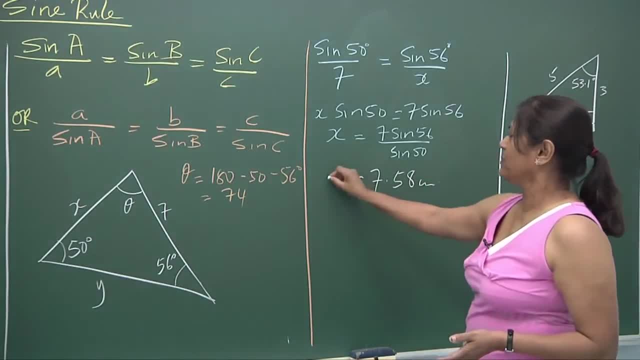 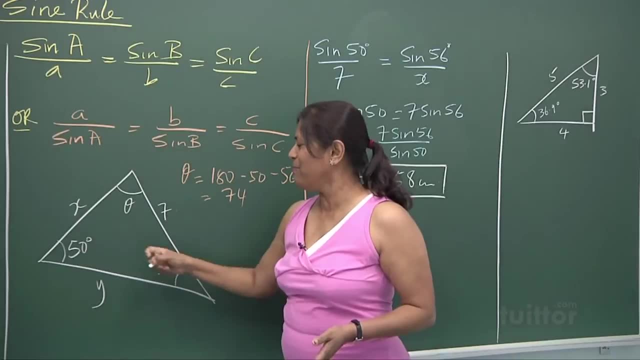 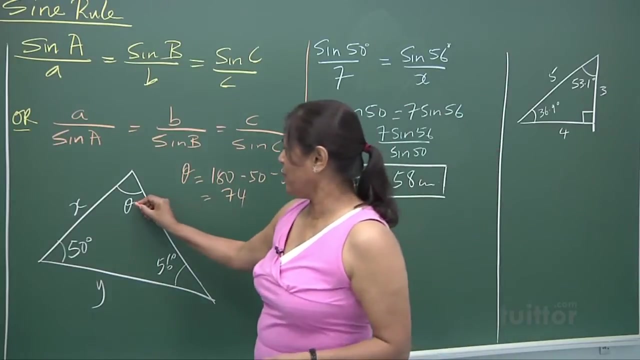 0.58 cm. so did i tell you, ah, it's going to be bigger than 7, right, because this angle is smaller than 56 degrees. now we gotta find out what is y, can you guess my dear? so we found theta to be 74. 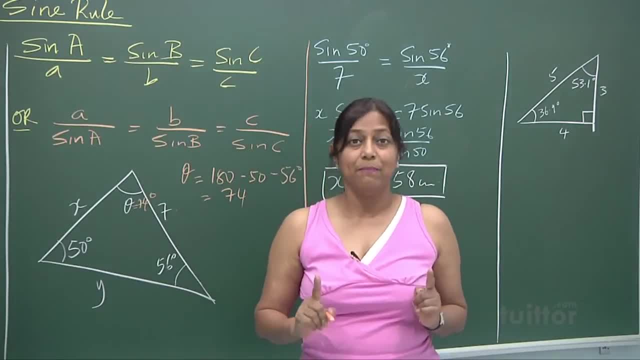 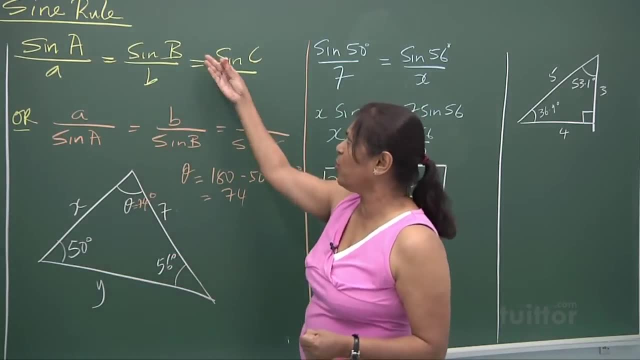 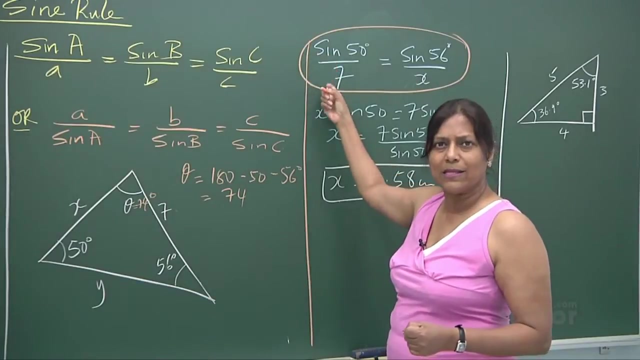 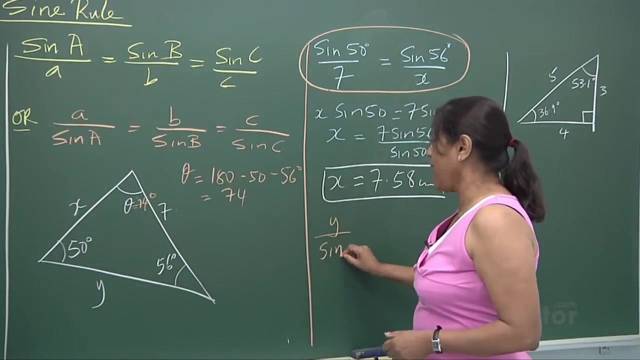 degrees. it's going to be bigger, right, because it's the biggest angle of the triangle. now we're gonna say a, but i told you that there are two ways of using this formula. i used this earlier on, all right, i used angle over the side. now i'm gonna try this way: y over sine, y over sine- 74 degrees. 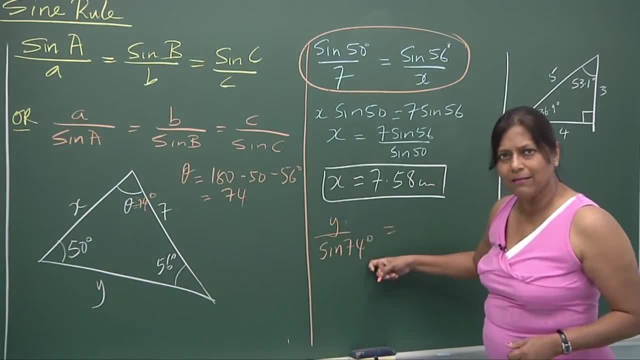 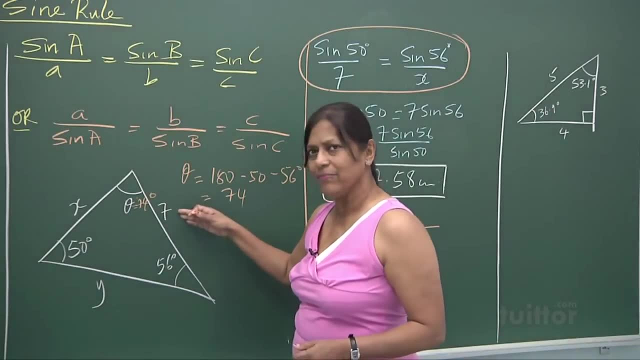 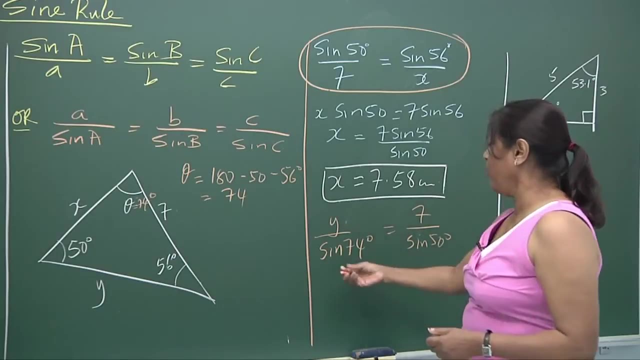 and if i put side over the angle, this should be side over the angle. please take note. and let me take what's given here. it is 7 over sine 50. all right, so you see it. we just all we need to do is bring your sine 74 here. 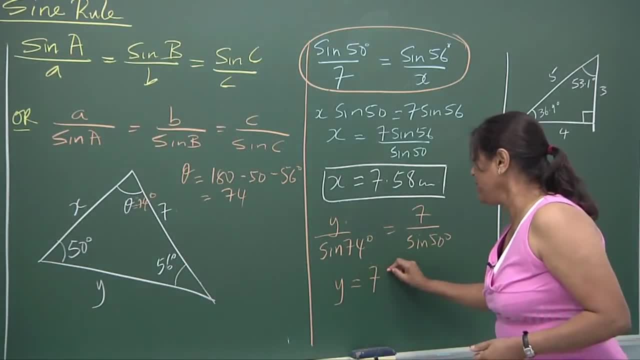 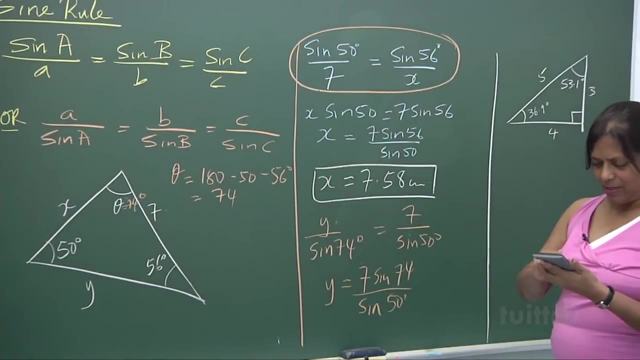 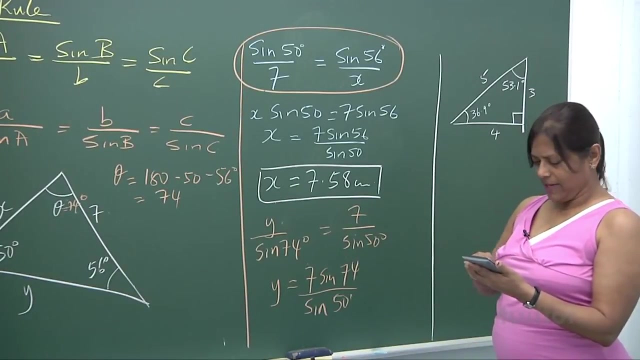 and you've got your y 7 sine 74, over sine 50 degrees. can you please help me there? yep, be a kind soul, get me the answer and let's see what you get. sine 74, all right answer divided by sine 50: all right, you will get this answer. you get 8.78. 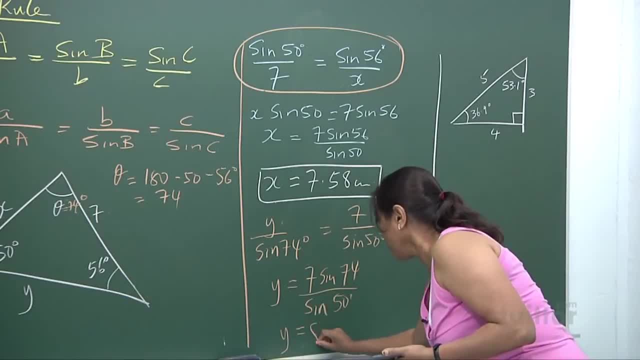 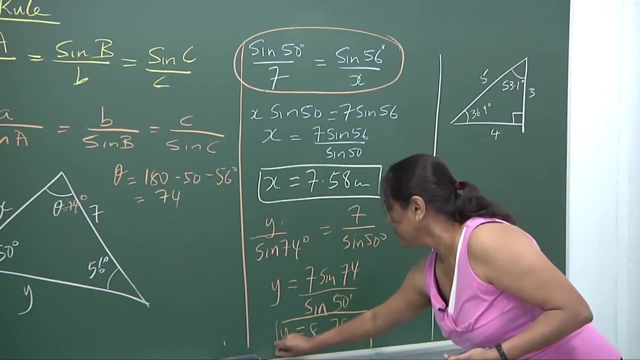 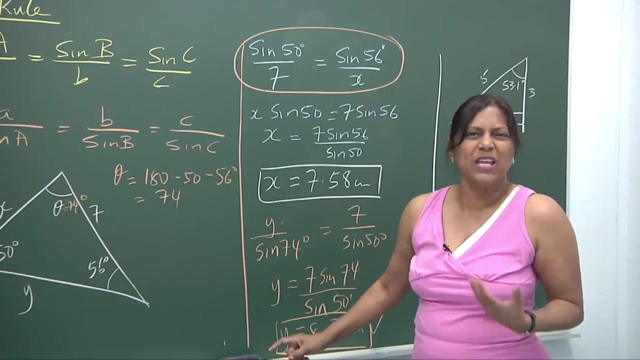 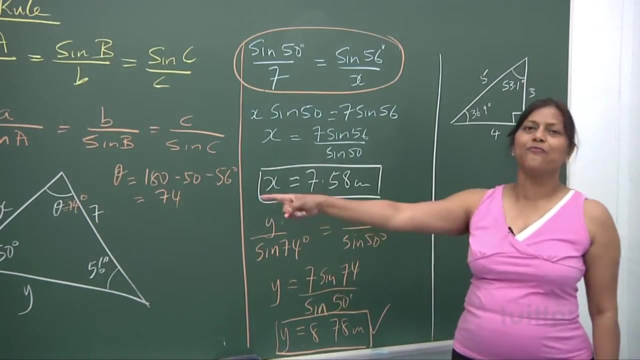 so your y is 8.78 cm. saw that this is the biggest side of the triangle. now, i'm sure you feel the level. sometimes when you do it, you can feel that internally. yes, i'm right, because it's a bigger sign and it it justifies it. okay now, but you want to find out. 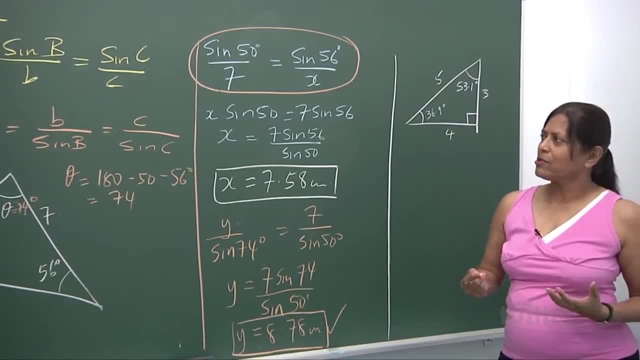 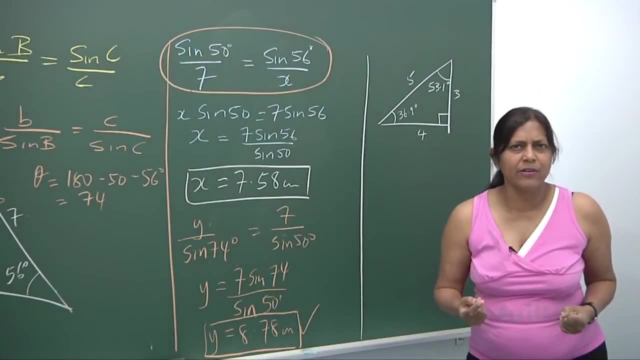 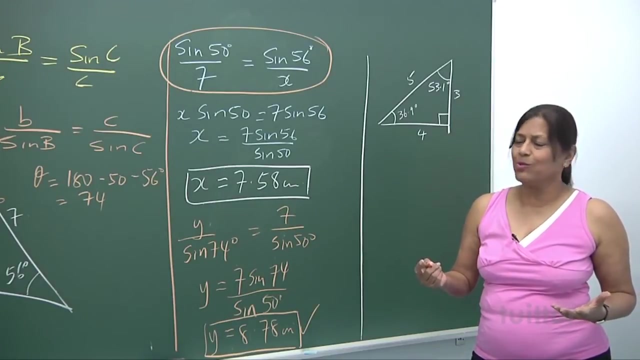 is sign rule only used for triangles that are for all triangles. is it for isosceles, is it for equilateral, is it for a skeleton or any triangle? all right, i would like to assure you. yes, it's used for any triangle. it need not be a right angle triangle, it can be. 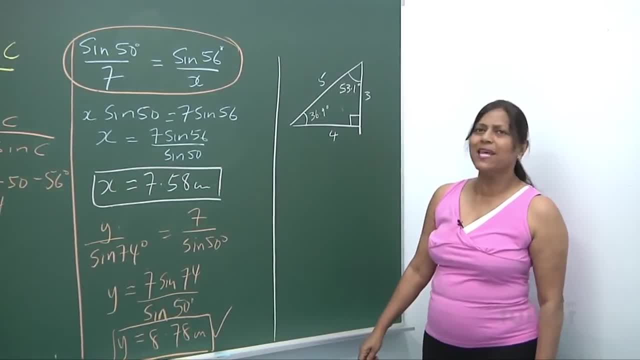 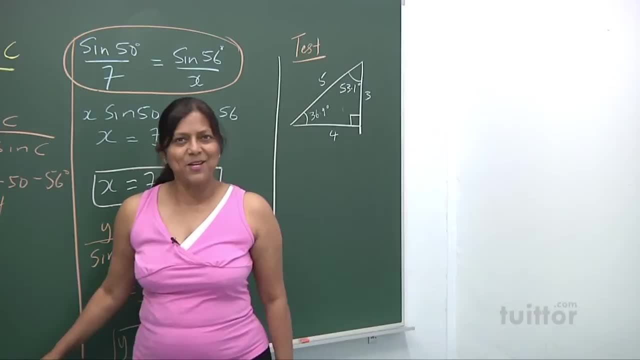 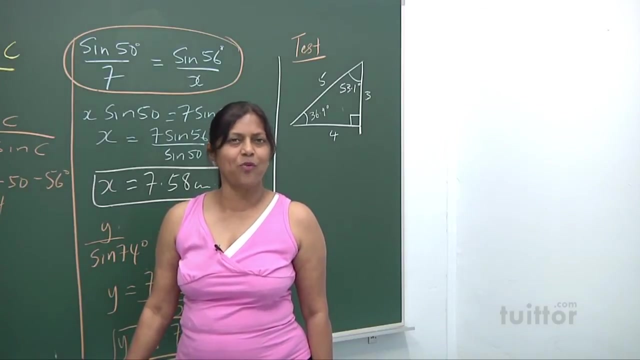 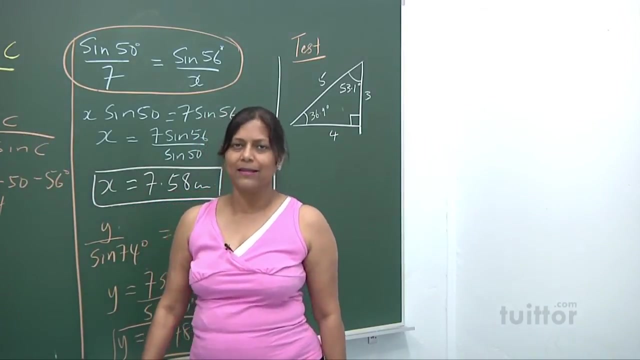 used for any triangle. let's do a little test. we take this. I came for a test, my dear. all right, I know you, young boy, young girl, you are just curious: how truthful is this formula? all right, you just learned the sign rule and I want you to know it's right. so let's do a little test. you're given this. 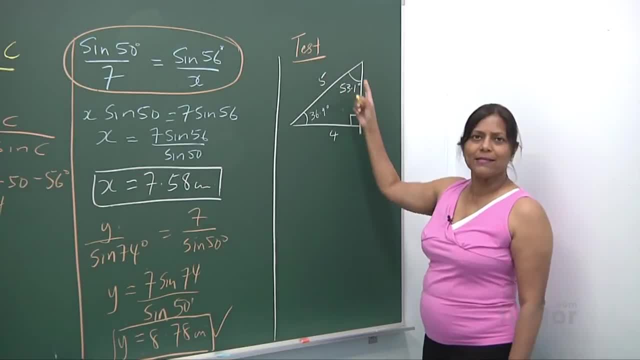 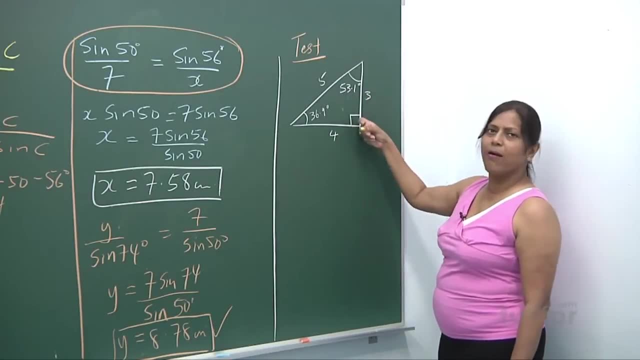 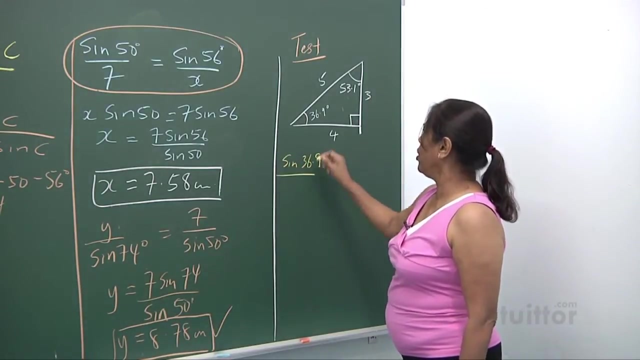 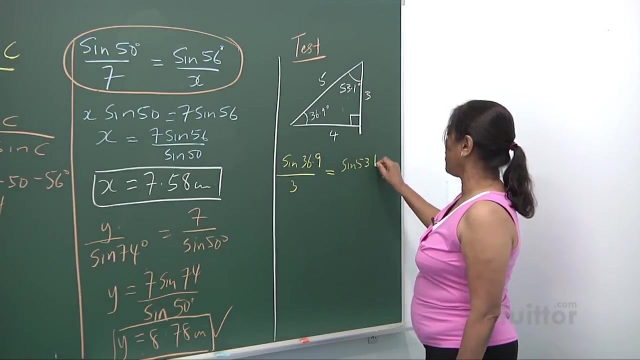 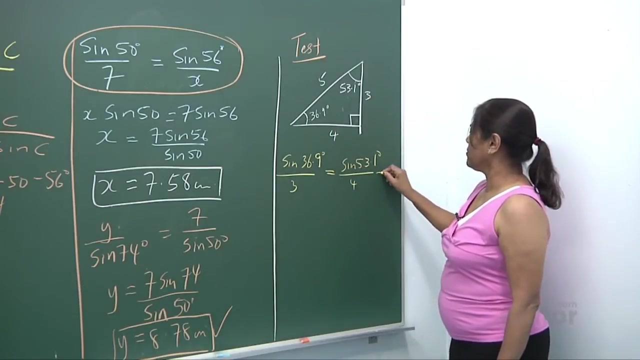 information: 3, 4, 5. it's a right angle triangle. we have 53 degrees. is 36.9, this 53.1, all right, this 90 degrees. so we said all right, we say sign 36.9 were facing 3 equal to sign 53.1 degree facing. look at it, facing for equal to. 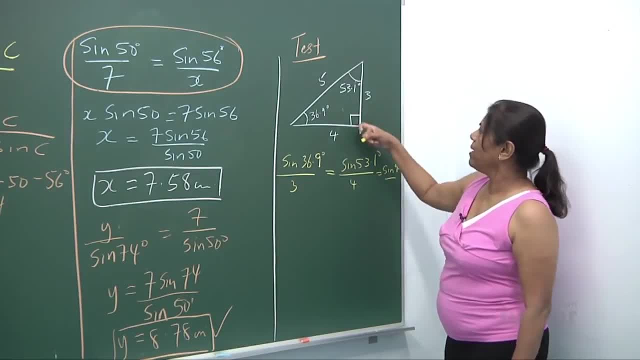 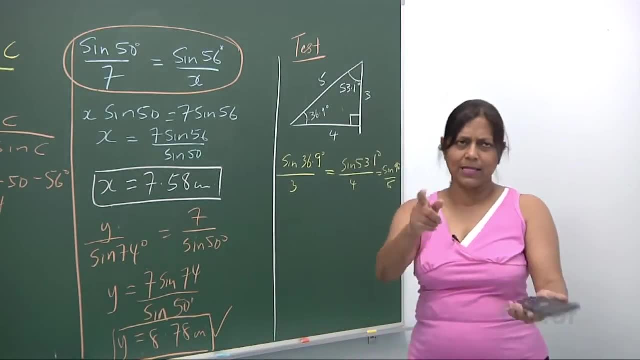 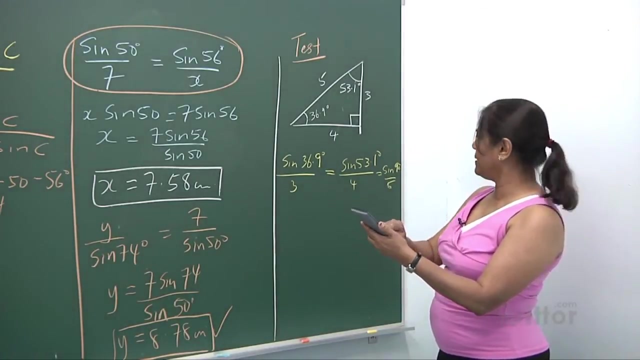 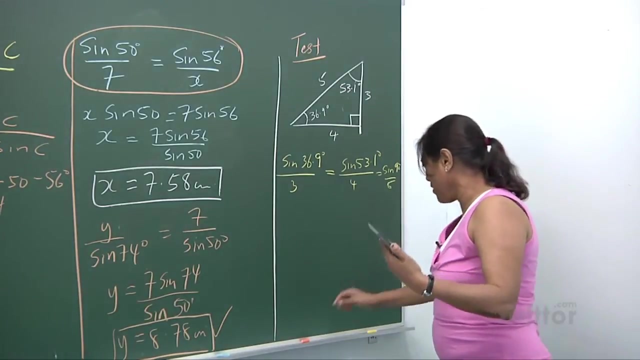 sign 90 degrees over 5. now please press your calculator. is the answer accurate? I just want you to test it. all right. what do you get? sign 36.9 divided by 3, what do you get? do you get the same as me- 0.200, right, if you got it. 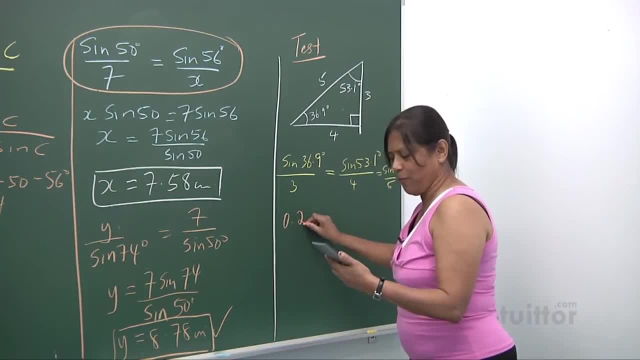 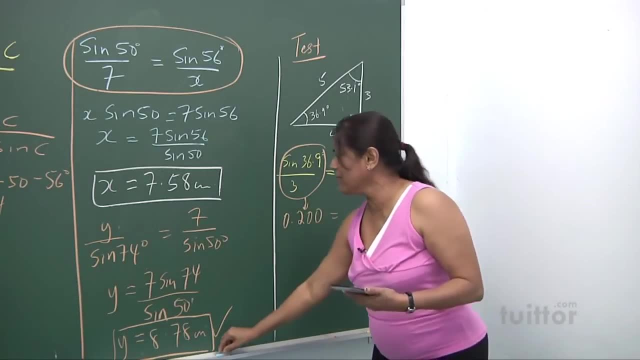 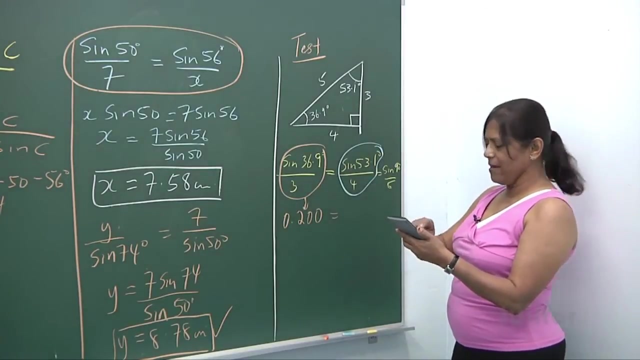 all right, let's put the two decimal place. all right, 0.200. that's the answer for this, mmm. what about the answer for this? we want to find out. is it 0.200, right? you press sign 53.1, close bracket 0.200 by 4 and you will get 0 point. 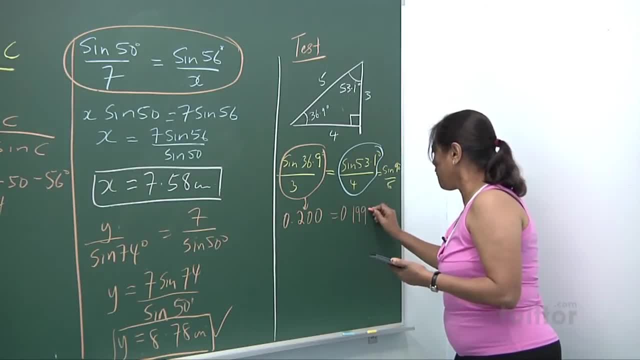 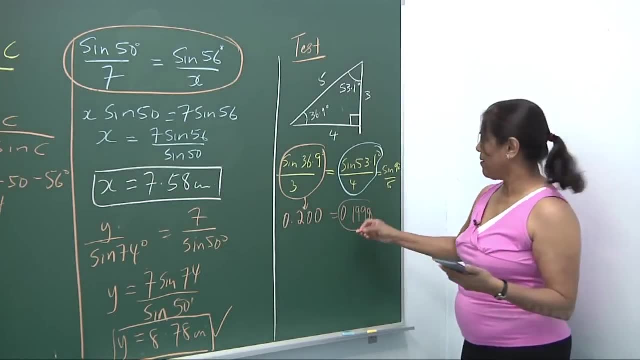 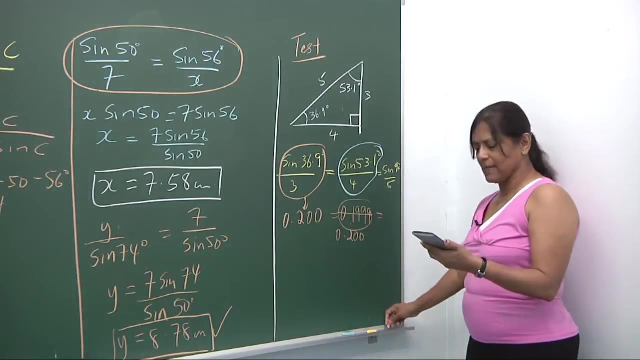 1999. all right, I just want to show you that if I were to round up, would this become that? so we're about there, all right, and I can just say rounding up, this will become 0.200. now look at the sign 90 divided: sign 90 divided by 4 and. 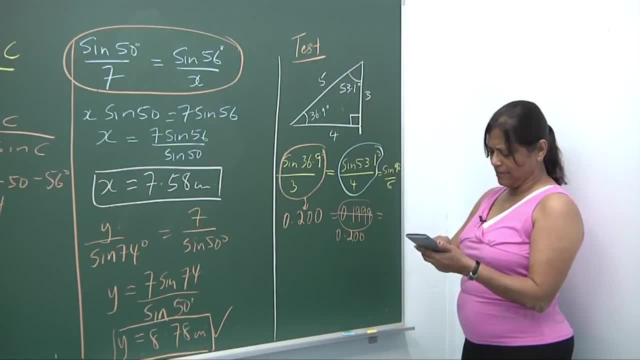 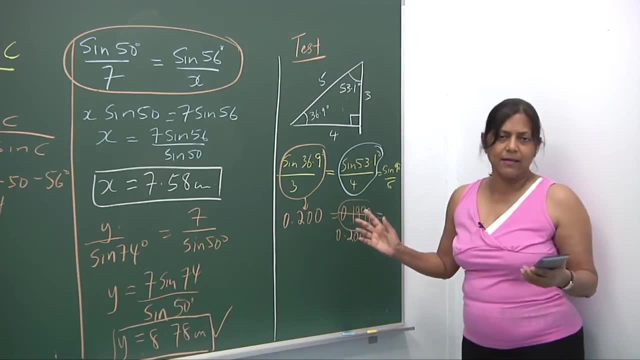 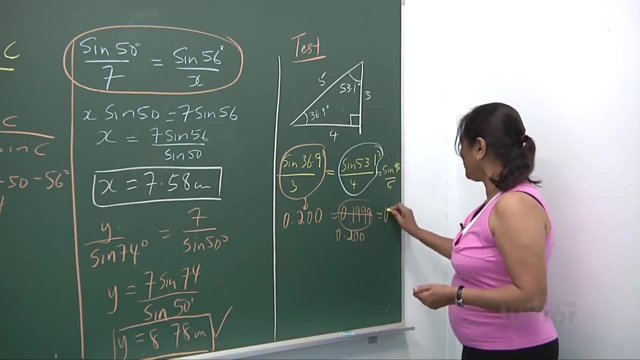 by 5,. all right, you know sine 90, it is actually 1, but I just want to make sure you know it. and you divide by 5, you get a 0.2,. all right, and 0.200,. so you say, hey, you are 0.2,. 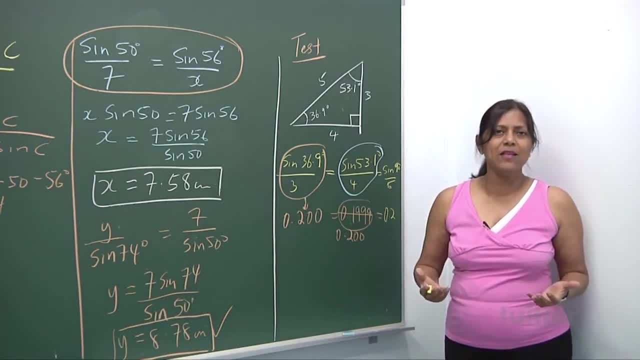 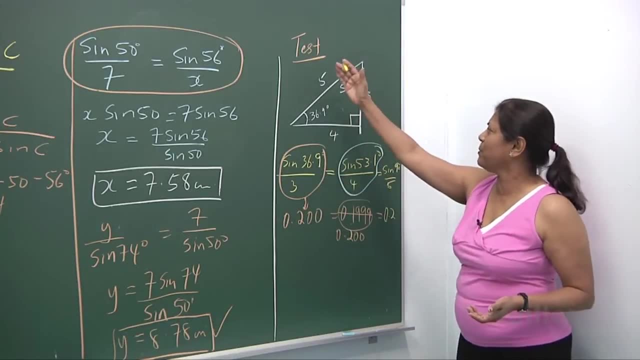 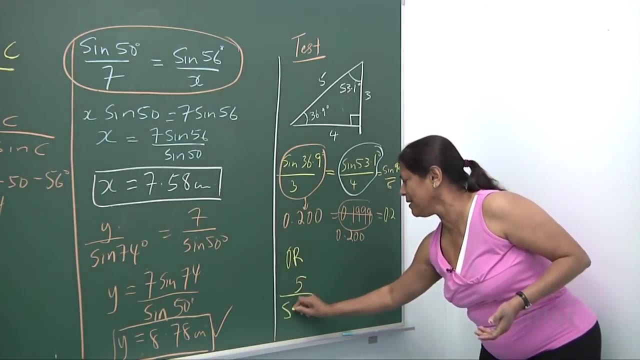 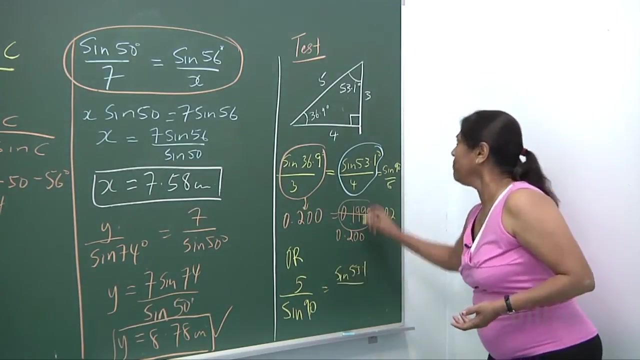 they are all there. so you can be very convinced from this example sine rule. they is there to stay. I can even tweak it. let's put sine over angle, okay. or I can say 5 over sine 90,, all right. I can say sine 53.1 over 53.1 over 4, and I can say sine sorry, sorry. 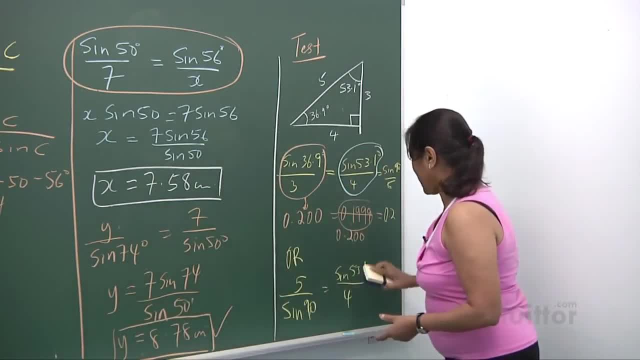 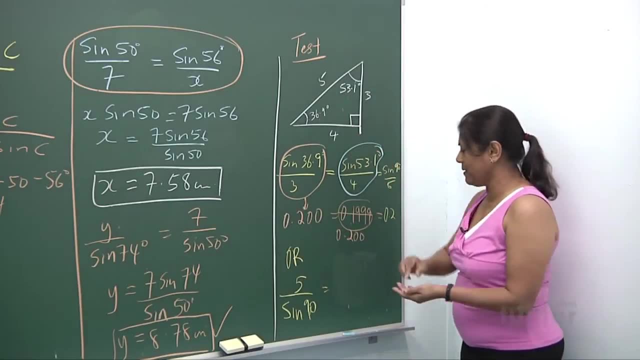 I was just a bit off. it's supposed to be this a side over the angle right, I said 5, over sine 90,, 3 over sine 36.9,. okay, you get 36.9, and I can say 4 over sine 53.1,. 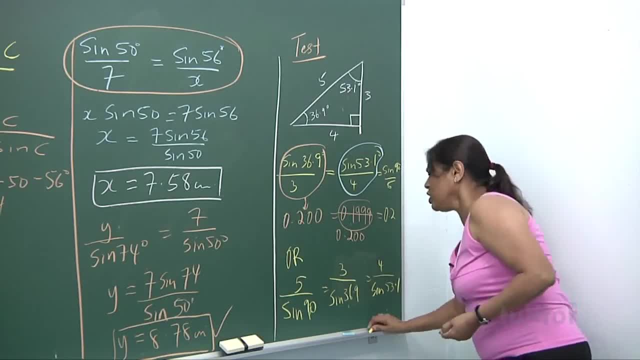 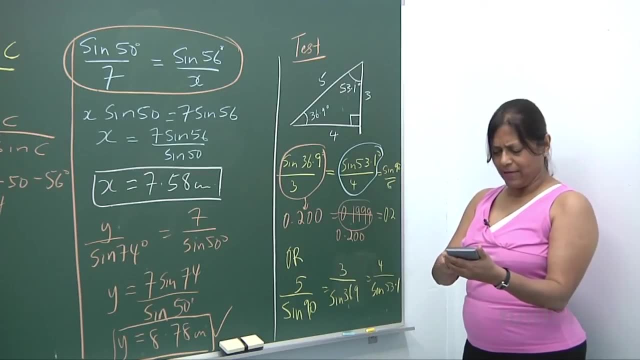 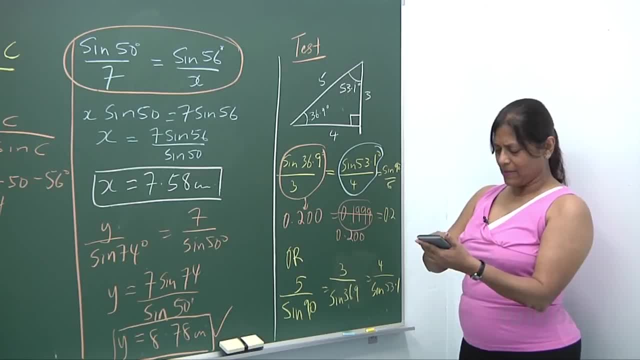 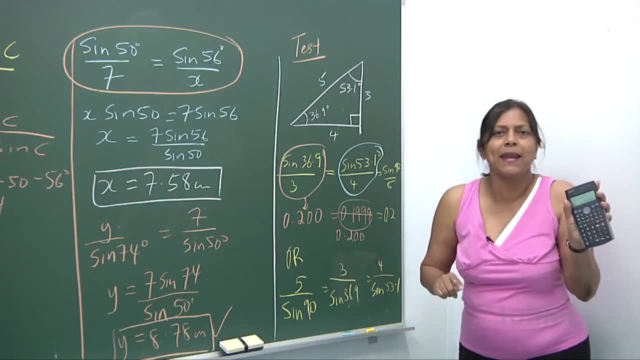 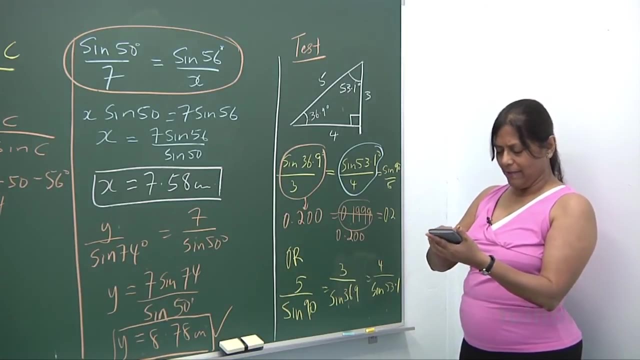 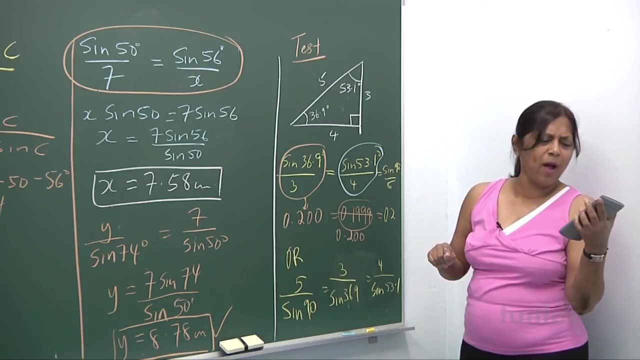 all right. you put 3 divided by sine 36.9,, 36.9,, do you get 5, I get 4.996,, 4.996, it's about 5, right. and when you get 4 divided by sine 53.1,, I get 5.001, it's all there. 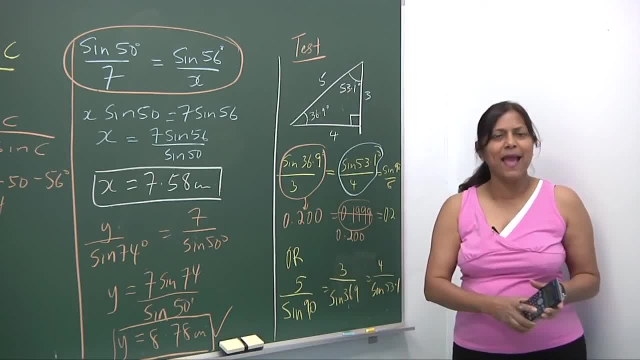 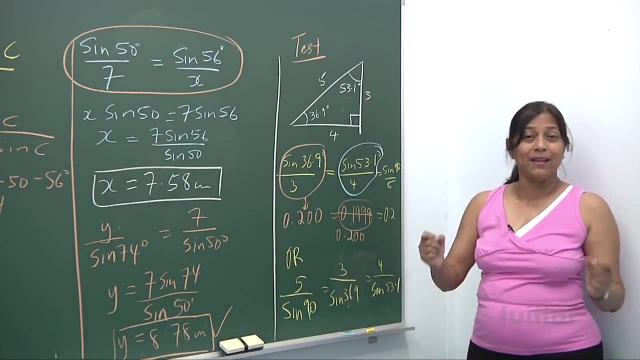 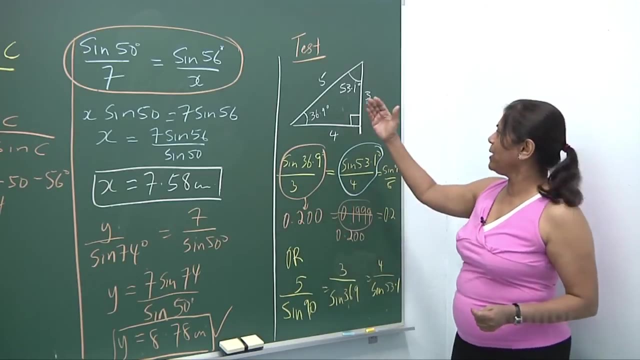 you know why the answer is not 100% accurate? because we, these angles were all surrounded, so that's why you don't get it 100% of accuracy, but they all show you. it is the truth that when you put an angle, 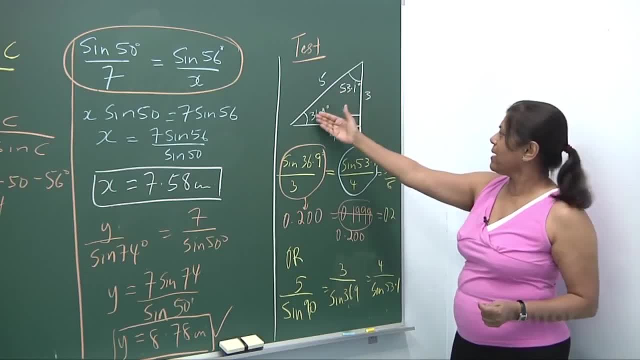 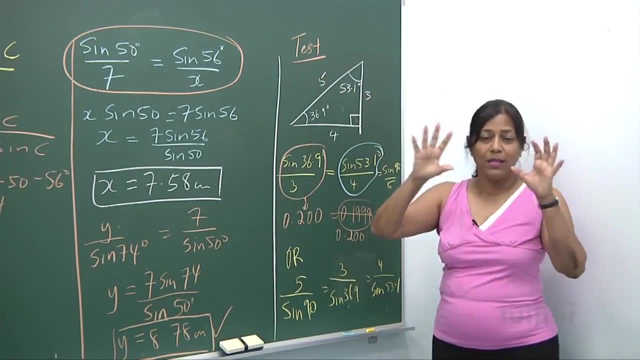 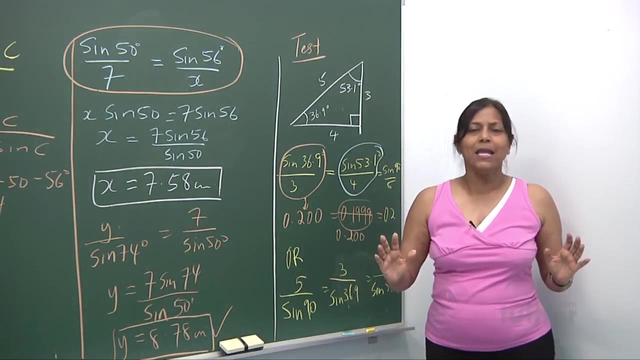 sine of an angle over the opposite side, sine A over A, sine B over B, sine C over C. they are all equal. the ratio of the sine over the sine. you get four sides for the three angles of the triangle. irrespective of whether it's obtuse, 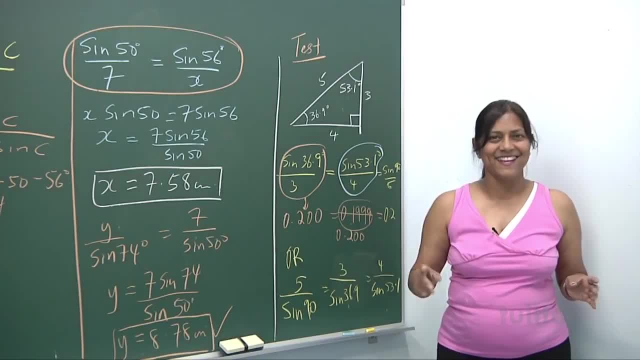 acute angle or whatever triangle it is. got your sine rule, yeah great.